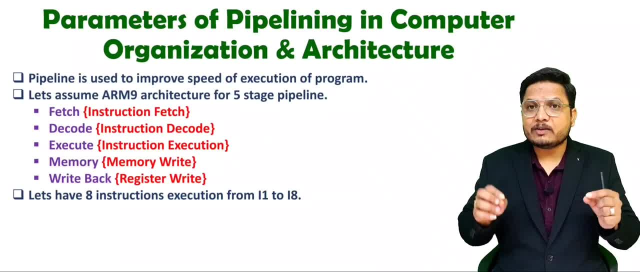 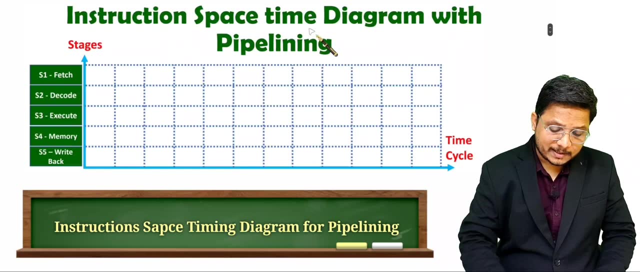 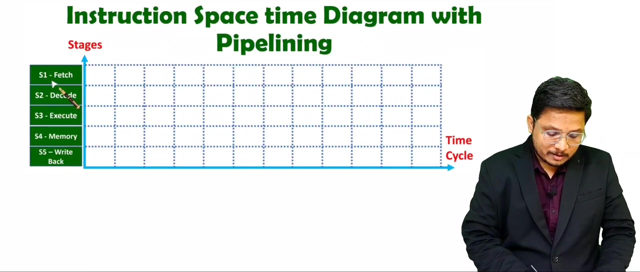 Right, So here, whatever answer that is there with you that you need to write in respected resistor over here. So that is how five stages are there And here we will be executing eight instructions. right, So let me explain you first how we will be executing eight instructions. So here, instruction space timing diagram that I'm going to explain you with respect to pipeline, And here you see we are having various stages: Fetch, decode, execute memory and write back. And with respect to time cycle, we will perform the instruction. 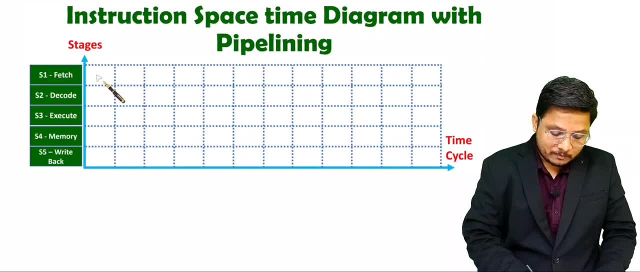 that execution with pipeline. So here in first cycle what will happen? Instruction 1, that will be having fetch operation. right In second cycle, instruction 1, that will get decoded in parallel with that second instruction. that will get fetched over here. 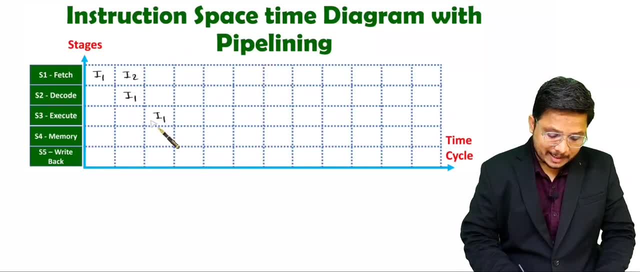 In third cycle. what will happen? First, instruction that will get executed in parallel with that. second instruction that will get decoded. and third is getting fetched. In fourth cycle what will happen? First instruction that will be going inside memory operation In parallel with that. second will get executed. 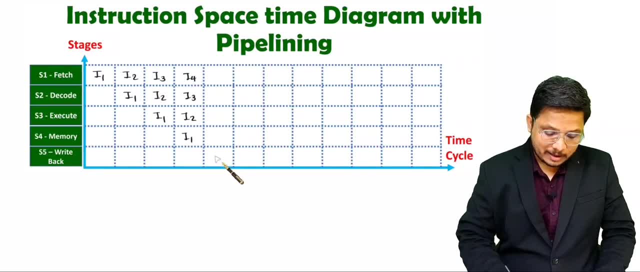 third will get decoded and fourth will get fetched In fifth machine cycle. what will happen? First instruction that will be having write back operation means you can say you have completed execution of first instruction. In parallel with that second instruction that will go inside memory write stage. 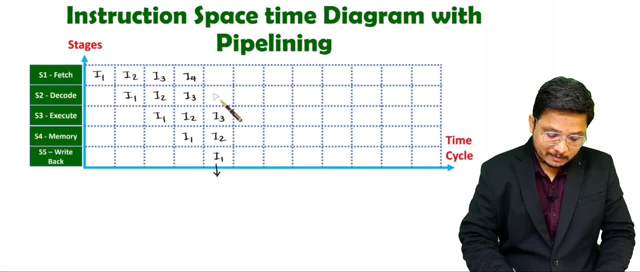 third instruction that will get executed over here, fourth instruction that will get decoded over here and fifth instruction that is getting fetched over here. In next machine cycle, what will happen? This I2, now that will go in write back stage, means that will come out of this CPU. 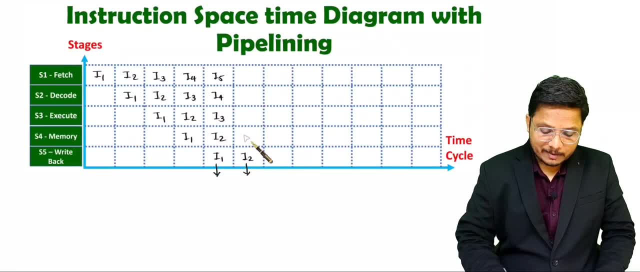 means you can say: execution is performed over here. In parallel with that, I3 will go inside memory stage, I4 will go inside execute stage, I5 that will be having decode operation and I6 that will get fetched In. next you will be observing I3 that is getting executed. 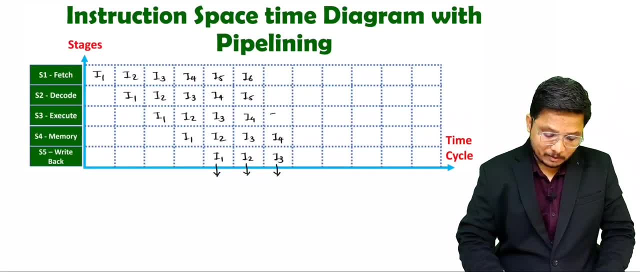 I4 that will go in memory stage, I5 now that will go in execute stage, I6 that will get decoded over here and I7 that is getting fetch over here In next machine cycle. this I4 now that will get performed over here. 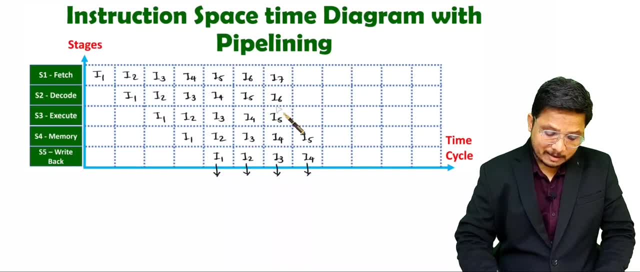 I5, that will go inside memory stage, I6, that will go inside execute stage, I7, that will go inside decode stage, and I8, that is then fetch over here and now we are having eight instructions, only right. so you see this i5. 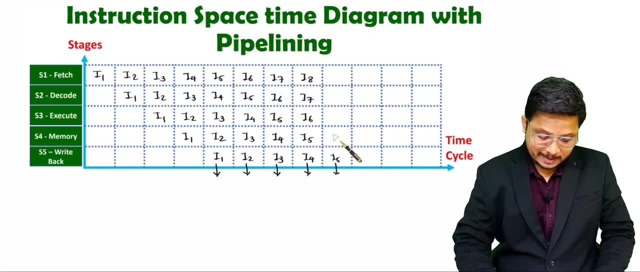 now that is getting performed over here. i6 that will go inside memory stage. i7 that will get execute over here. i8 that will get decoded over here in next cycle. i6 that will get performed. i7 that will go inside memory stage. i8 that will get execute over here in next cycle. i7 that will 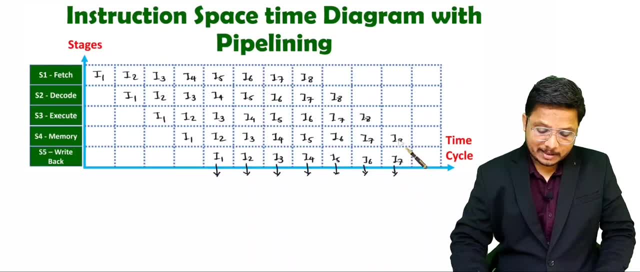 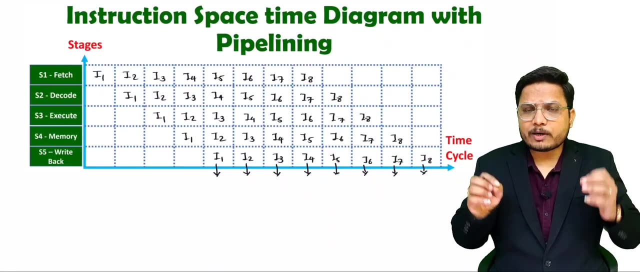 get performed means write back i8 that will go inside memory stage and, in next cycle, i8 that will get performed over here. so our program, which was having eight instructions, you see now that is getting completed over here right now. here, my dear students, we need to understand. 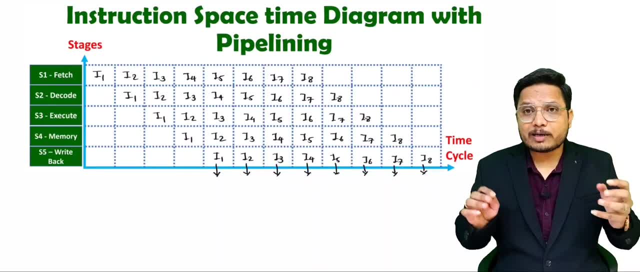 how exactly things are happening. so first of all, you will have to understand one thing: how much time pdr that is taken over here with pipelining right, and how much time you will have to take over here with pipelining right, and how much time you will have to take. 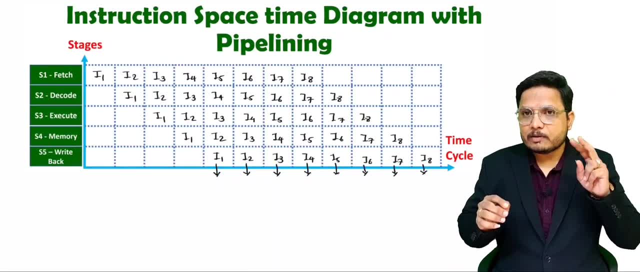 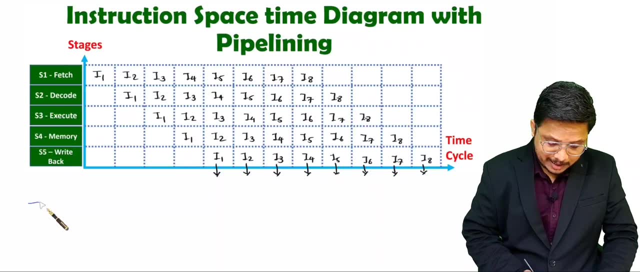 over here with pipelining, right, and how much time you will have to take over here with pipelining. that is possible without pipelining. the reason is, these two parameters are very essential, right? so as if i want to calculate how much time pdr that we need to have without pipelining. 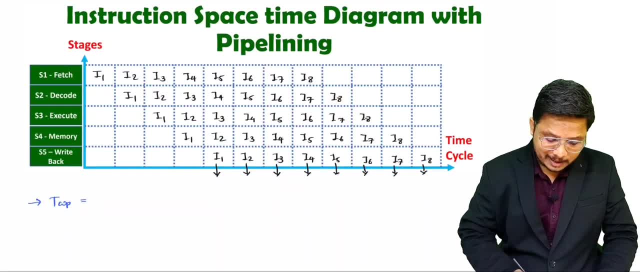 then you will be observing: how many instructions are there? eight instructions are there. let us say number of instructions: are n into how many stages are there? so five stages are there. let us say number of stages, that is k, so n into k and for one stage as a. 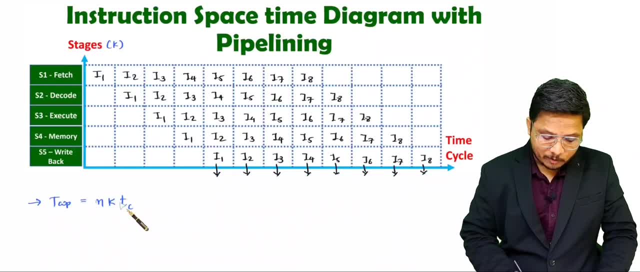 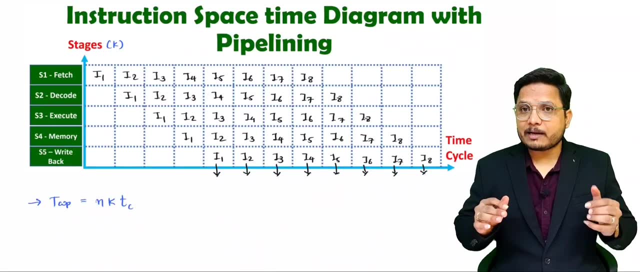 as if i say cycle time, pdr, that is tc, then without pipelining, n, k tc, that will be the time pdr. now let us try to understand how much time pdr that we need to have with pipelining right. so if you observe here, my dear students, for first instruction, execution, you will be observing how much time. 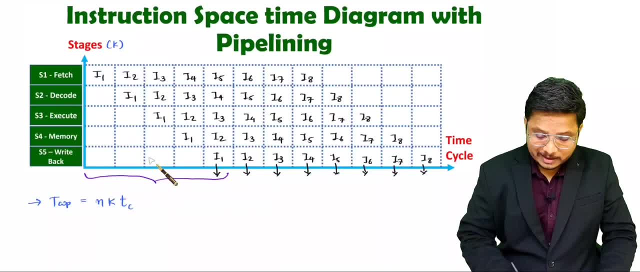 pdr that we need to have. so 1, 2, 3, 4, 5, 5 stages that we need to have right and how many stages are there? k number of stages are there and how many stages are there? k number of stages are there. 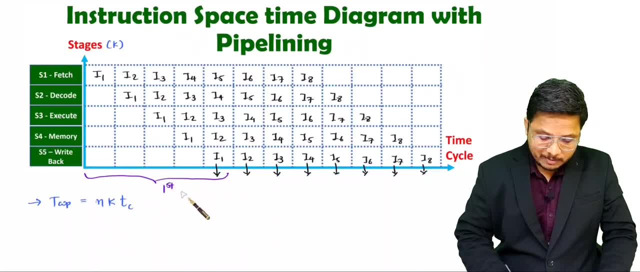 so for first instruction it will be taking k cycles right, and for n minus 1 instructions. how many cycles that it will take for each instruction? you see now it will be taking one cycle only. so for n minus 1 instructions it will be taking n minus one cycles. so here, my dear, 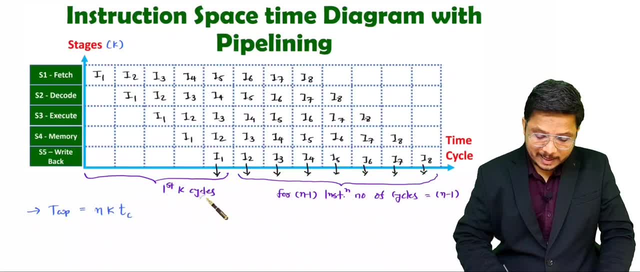 students. for first instruction it was taking k number of cycles and for rest n minus one instruction It was taking N minus one cycles, right? So how much time period that is there with pipeline? So for pipeline structure time period will be K plus N minus one, right? 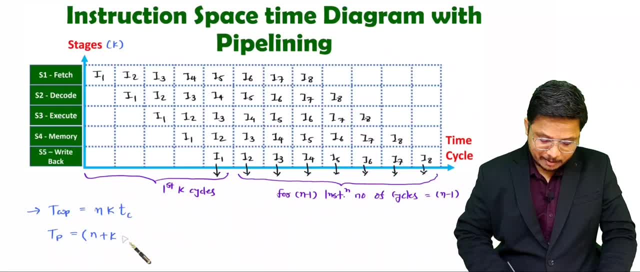 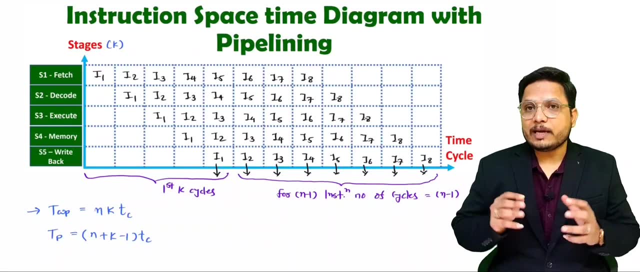 So I can say N plus K minus one into TC. That is what the time period that is there with pipeline structure, right? So here, technically, if you observe for eight instructions without pipelining how much time period that it will have took eight into five means 40 cycles, right. 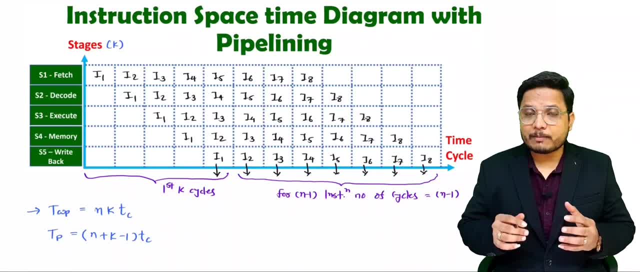 And with pipelining, how much time that you will be taking over here with pipelining. You see, K is five plus N means eight, means five plus eight. 13 minus one means 12 cycles, right, So you see, one, two, three, four, five, six, seven, eight, nine, 10,, 11,, 12.. 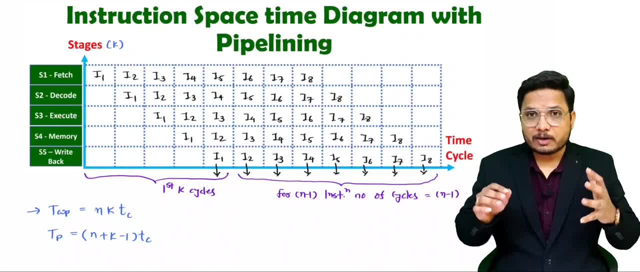 So 12 cycles that we need to have to have execution of instruction with pipelining along with five. So that's what we're going to do in the next two stages and without pipelining it will be taking 40 cycles, right. 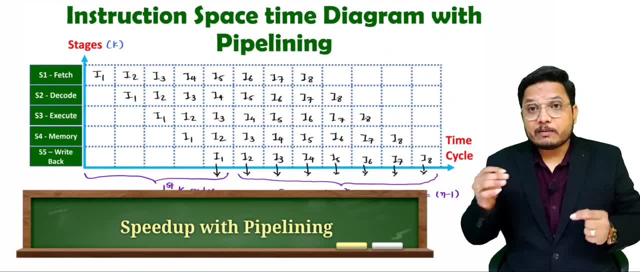 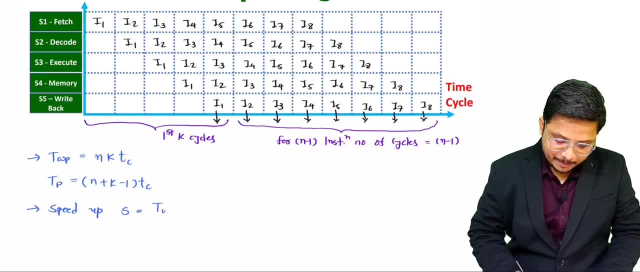 Now I'm going to explain you speed up of computer with pipelining or without pipelining. So speed up is how much? speed up is time period without pipelining divided by time period with pipelining. time period without pipelining. 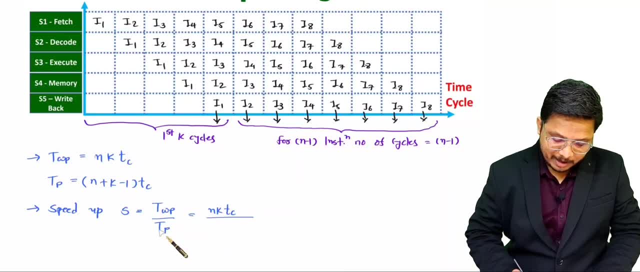 That is N into K into cycle. time period divided by time period with with pipelining, That is N plus K minus one. Okay, One into TC. this time period of clock cycle that is getting canceled, So speed up- will be N into K divided by N plus K minus one. 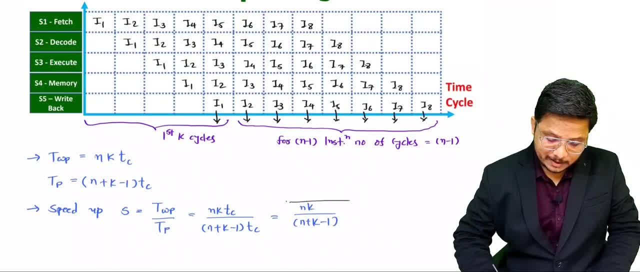 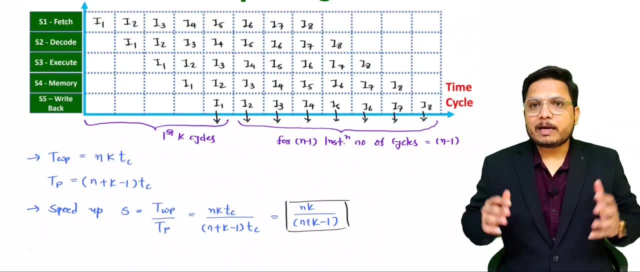 So this formula, that is very essential, You must have to remember this speed up- that is N K divided by N plus K minus one. Now, my dear students, I'm going to explain you how we can identify throughput. So first of all, you should know what is throughput. 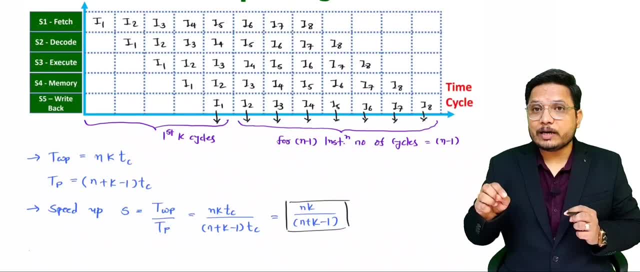 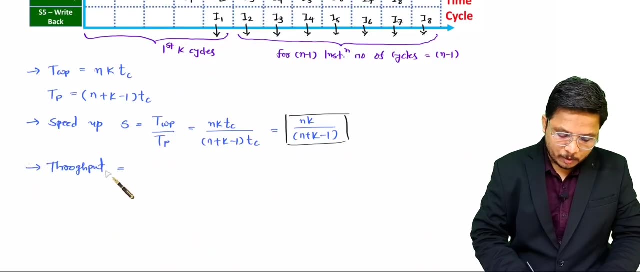 See throughput. It means how many instructions that is getting executed with respect to time, right? So when you want to calculate throughput that explains you how many instructions that is getting executed with respect to time. Let me explain you how to calculate that. So throughput means number of instructions with respect to time. 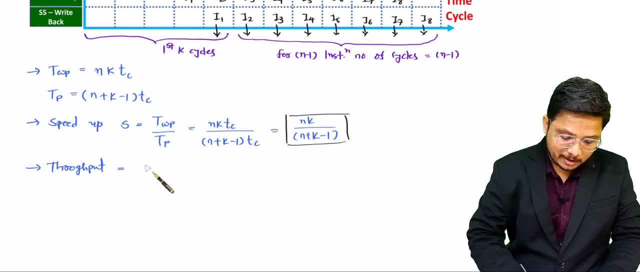 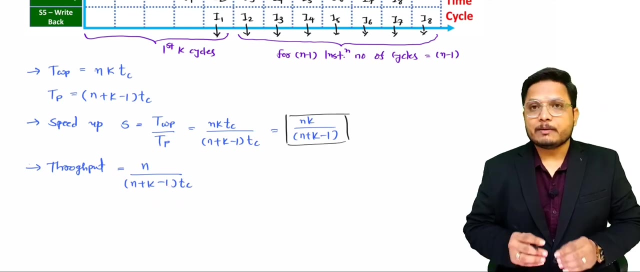 So how many instructions are over here and number of instructions are over here and how much time that we need to have with pipeline structure. So N plus K minus one One into TC. So throughput over here, that is N divided by N plus K minus one into TC. 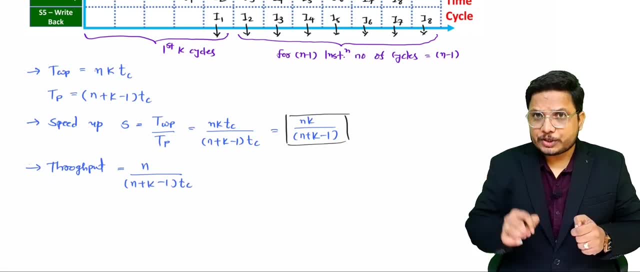 Many of the times you will be observing, you will be asked with this question right In examination, So they will be asking you throughput. So first of all you should know what is the meaning of it. It is number of instructions executed with respect to time right. 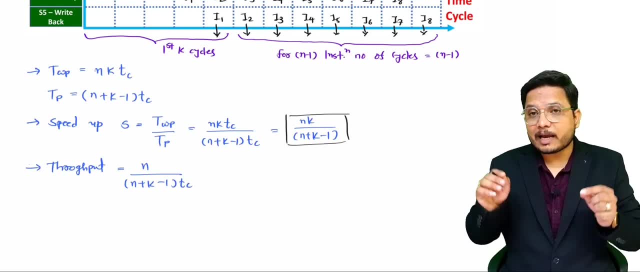 So that will be N divided by N plus K minus one, into TC. but here sometimes they may not give you, It is number of instructions, right? So at the time, how to identify throughput. So you should know, my dear students, when you have not given with that number of instructions. 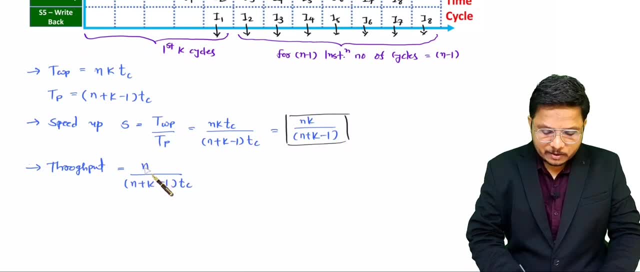 at that time you'll be observing this number of instructions. Those are considered as infinite, So infinite by infinite. that is getting canceled as we neglect K minus one over here. So throughput will be one divided by TC and you can say: this is ideal throughput. 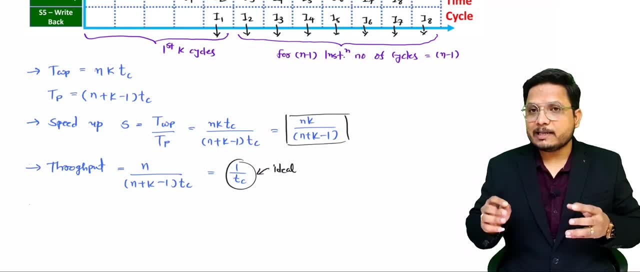 So many of the times I have seen, They will be asking you this question In that number of instructions may be given to you. In that case, you will have to use this formula and divide by N plus K minus one into TC, right. 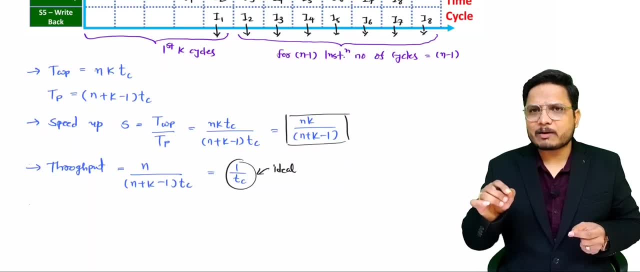 But as if number of instructions are not given, then you'll have to simply calculate that as per one by TC, where TC is time period for one operation or one stage. right Now I'm going to explain you how we can identify efficiency, and that is also referred as utilization. 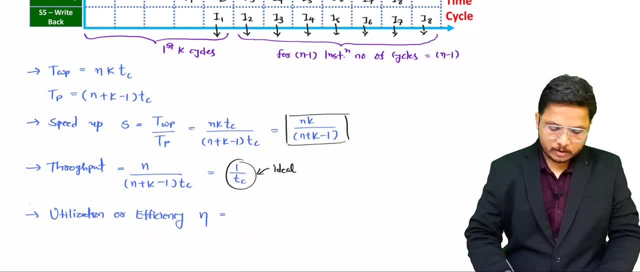 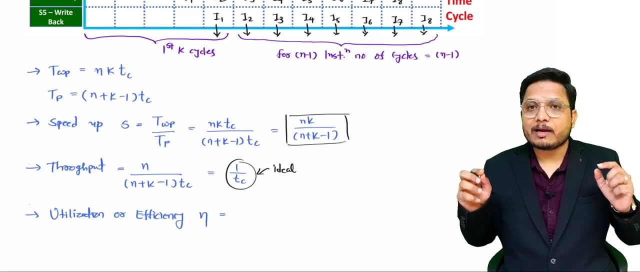 of CPU, Right? So what is the meaning of efficiency or utilization? See, utilization means when you execute any program, at that time all the blocks which are there inside CPU is it getting utilized? If it is utilized, then you can say: 100% efficiency is there. 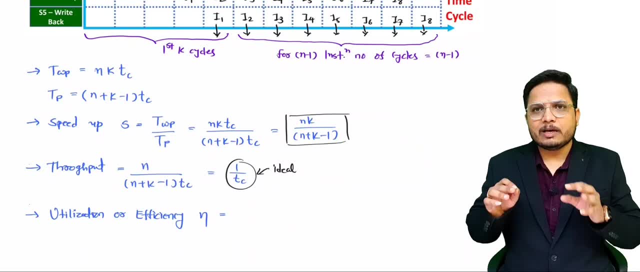 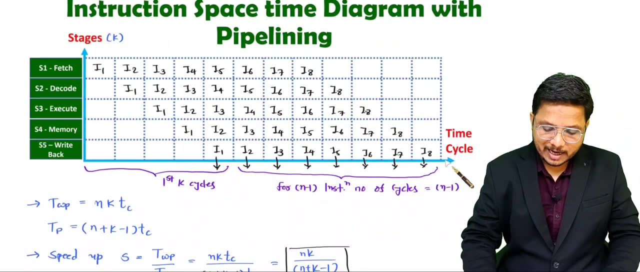 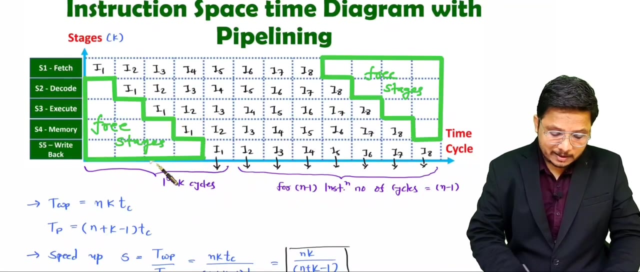 So ideally you can say 100% efficiency is there, but practically you can say all the blocks are not utilized. You see over here in problem. Also, I have shown you pipeline structure. I have shown you pipeline structure Right. But in that if you observe during five stage pipeline execution- these are the stages which 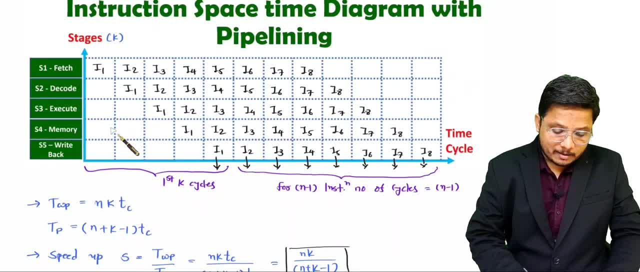 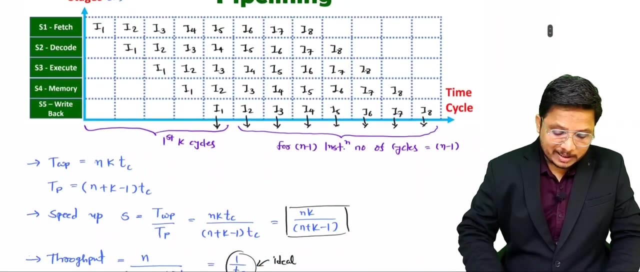 are not utilized. You see, right, And you'll be observing these are the stages that is getting utilized over here. right, So how to identify efficiency, total number of blocks and utilized blocks ratio. right So, how many that we have utilized. 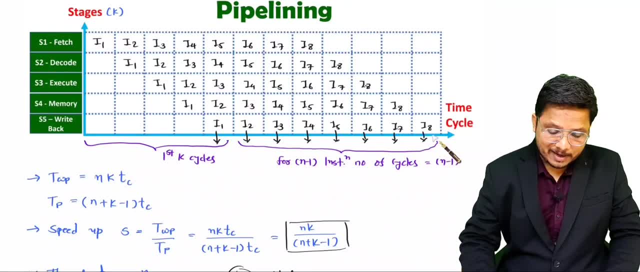 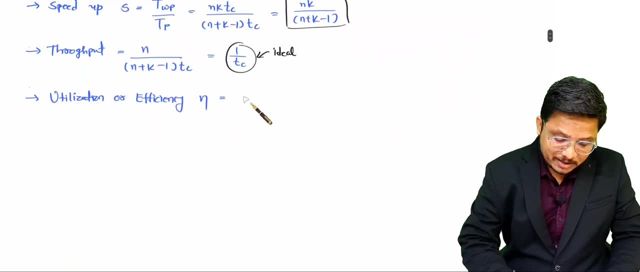 So here, K stages are there, Right? These are the instructions that we have executed. So K into N, that is what number of stages that we have utilized over here. So let me mention that N into K, those are the stages which we have utilized over here. 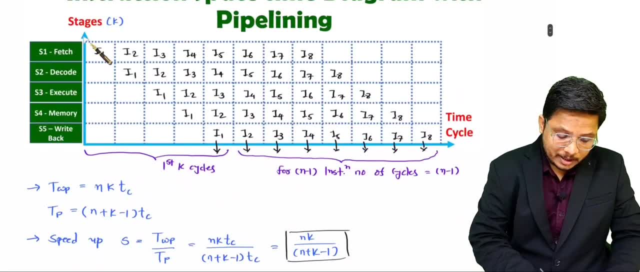 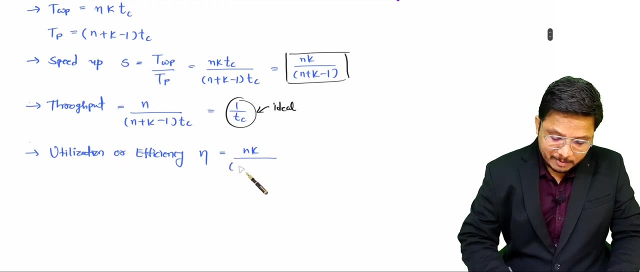 And how many total stages are there. So here you see, total stages are that many, And in that, this is what: vertically we have K and horizontally how many cycles that we have K plus N minus one, Right? So? So the denominator will be having N plus K minus one and into K, don't forget this right. 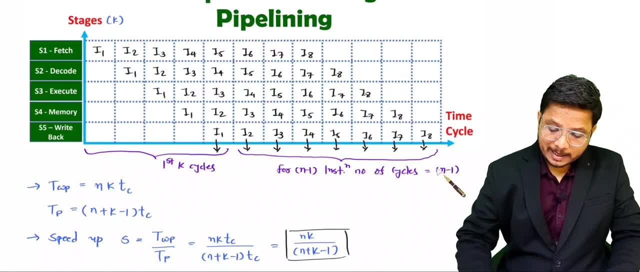 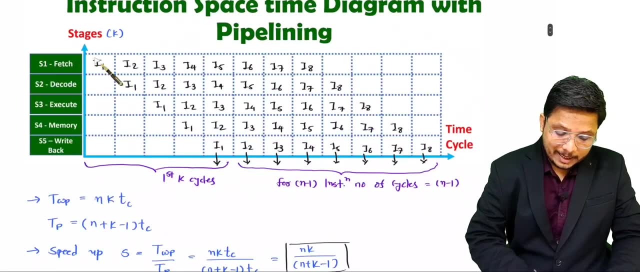 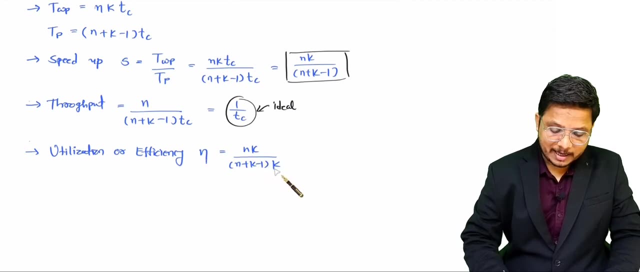 You see total stages, that is K plus N minus one into K, right? That is what total stages over here and utilized are K into N instructions, right? So you can say efficiency, that is N, K divided by N plus K minus one divided by K. And if 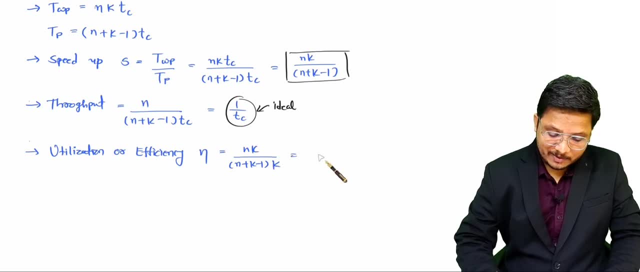 you observe here this K and this K. that is getting canceled. So I can say N divided by N plus K minus one. Here, my dear students, there are some questions that may come based on relation of speed up and efficiency. So if you observe both formulas, both are almost same. only with S you have to multiply.